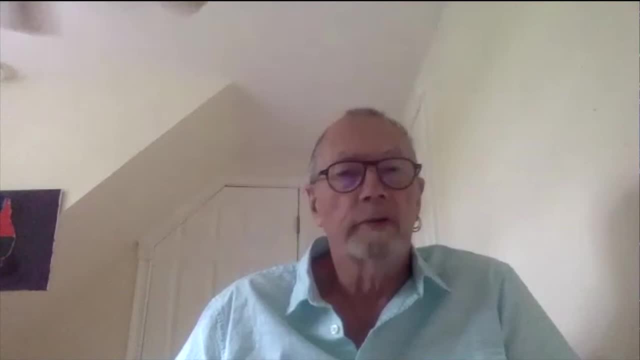 the language will tell you what are the grammatical sentences of this language. The formal system itself will pick out a subset of those sentences, those which are provable in a certain sense. Mechanisms of proof come in various kinds, but usually, when Gödel's theorem is discussed, it's assumed that we're. 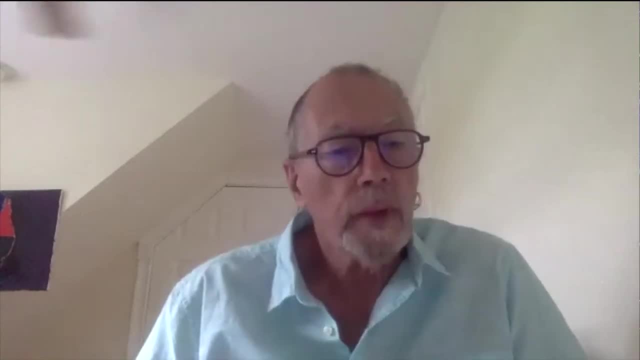 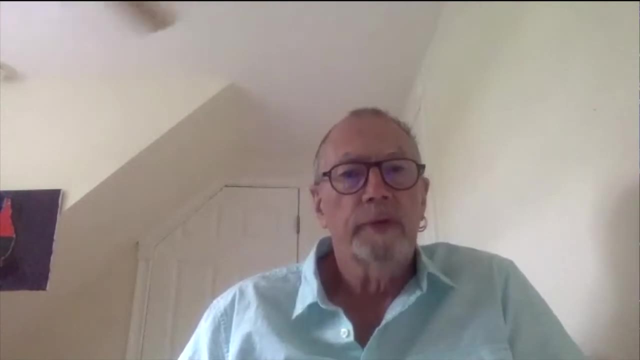 dealing with an axiom system of some kind. So in an axiom system, you pick out a subset of the grammatical sentences as axioms. Those are the things which don't need any allegory. So in an axiom system, you pick out a subset of the grammatical sentences as axioms. Those are the things which don't need any allegory. 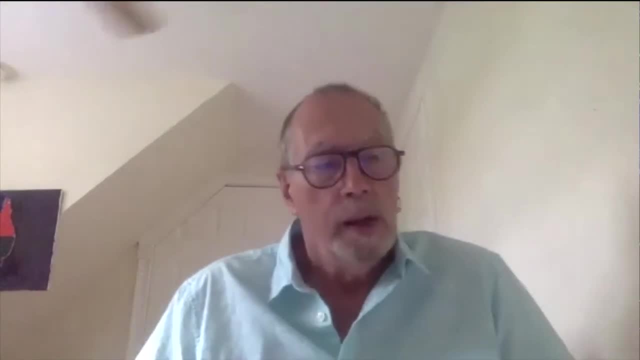 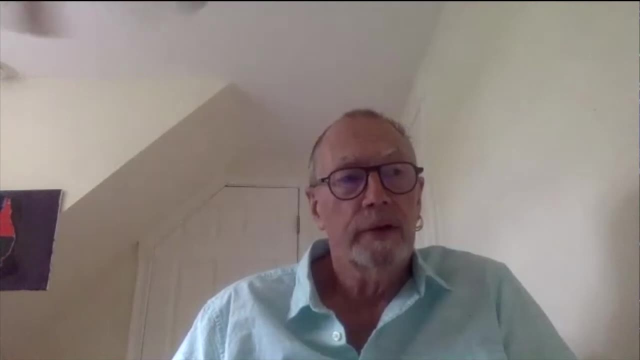 kind of proof. They're just the givens. Then the formal system will come with an inference engine. that is a way of inferring conclusions from premises, Usually in the context of Gödel's theorem. it's assumed to be classical logic. but 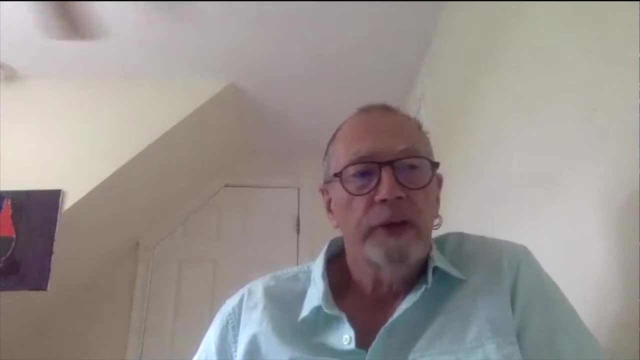 that's not necessary for a formal system in general. It's actually not even necessary for Gödel's theorem, but it's an assumption that's usually made. Given that you've got the axioms, and given that you've got a logic, then the 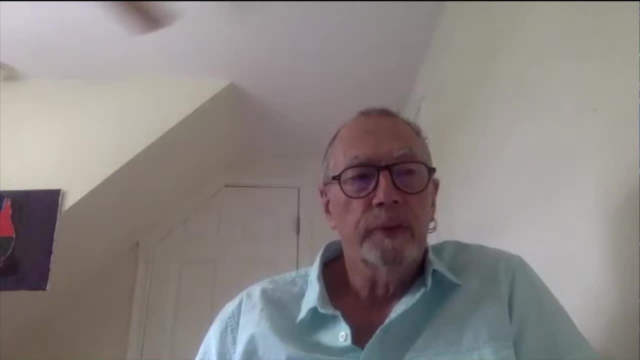 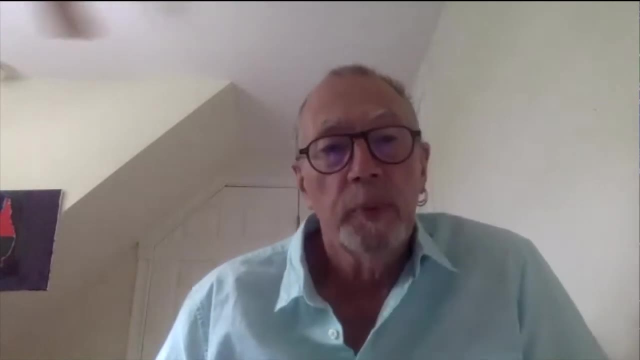 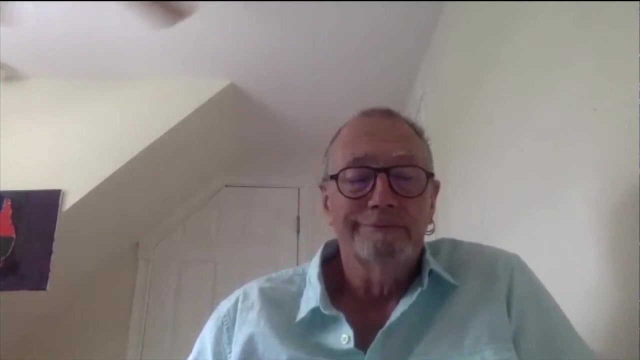 theorems of this formal system are simply the things that you can infer from the axioms by using the inferences permitted by the inference engine you're using. Given the axioms, you can apply the rules of inference to get some more theorems, and then you can apply the rules of inference again to get some more theorems. 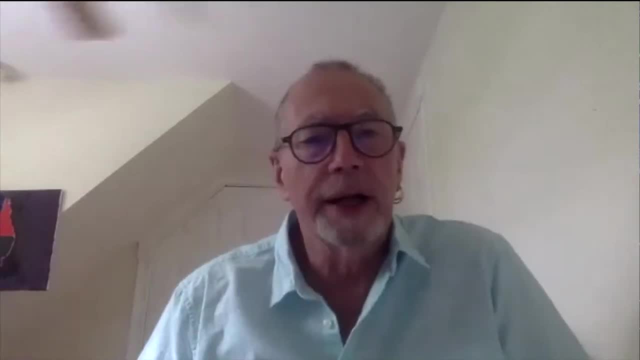 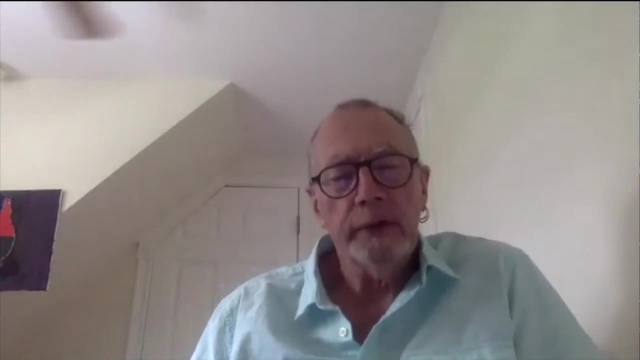 And so on, indefinitely. You can do this and generate an infinite number of conclusions. What this means- and so that's the kind of very simple level of abstraction. but what this means is that, given a bunch of axioms, what you can do is you can keep applying the 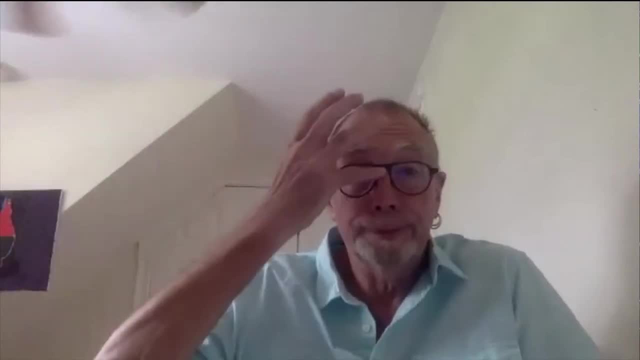 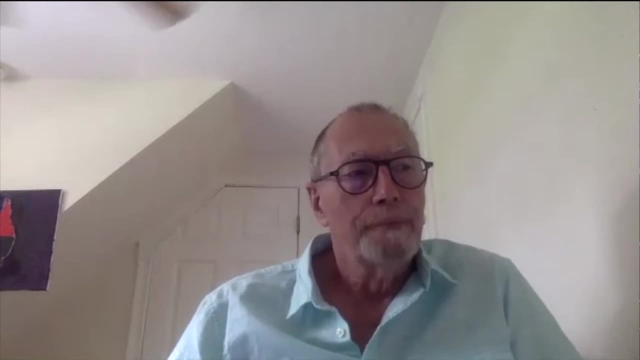 inference rules and so generate a whole bunch of theorems. So you generate an infinite number of theorems. You may have no particular way of telling whether a theorem is going to be produced in the end or not, but at least you can be sure that if you keep applying the rules indefinitely, 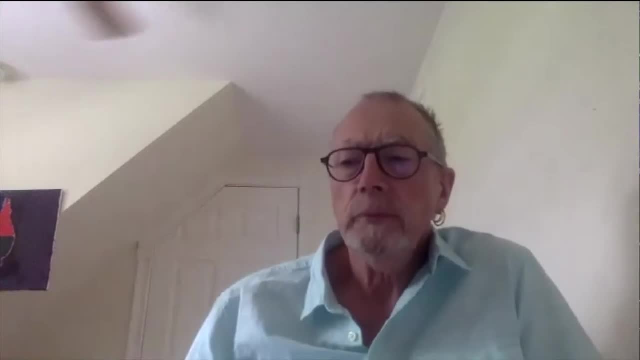 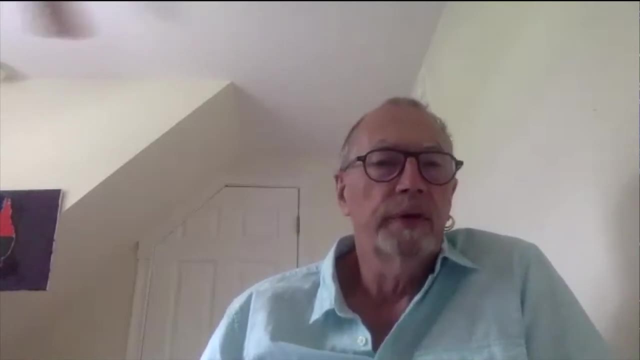 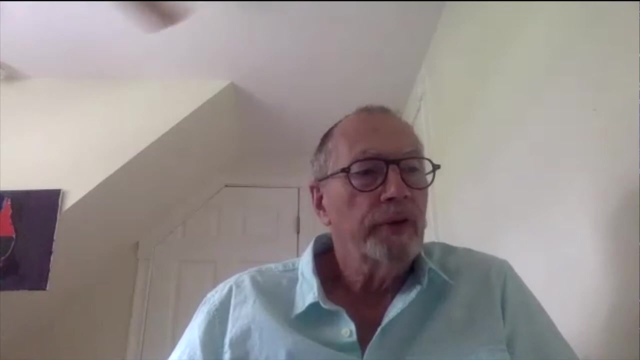 you're going to generate all the theorems, because that's how it's defined. Now, the more general setting of this is something called recursion theory, which is a theorization of effective procedures, And so. So The simplest level of decidability in recursion theory is: a set is decidable if there's an. 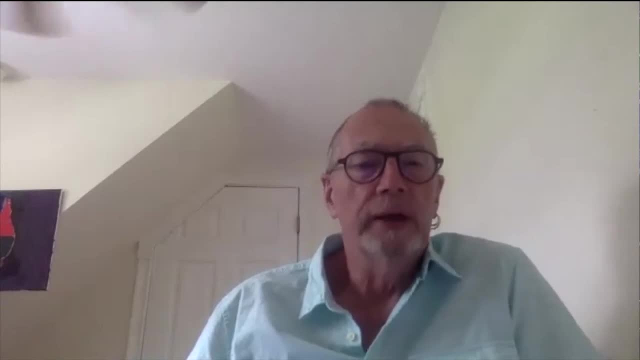 algorithm which will tell you whether something is in this state or not. So a very simple theory might be such that there's an algorithm to tell you whether something is a theorem, But generally speaking that's not going to be the case with formal theories. 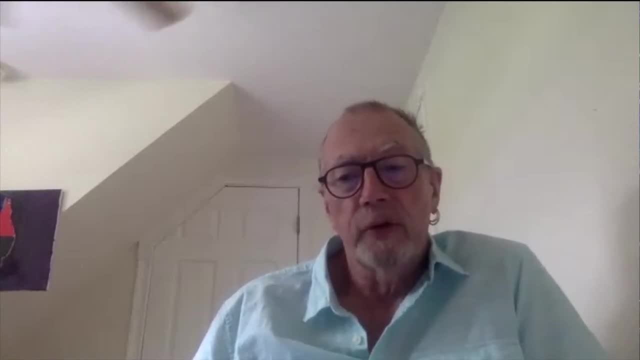 As I say, you may not have a theory, You may not have an algorithm which tells you whether something is or is not a theorem, But at least you know you can kind of turn out the theorems in this sort of step by step. 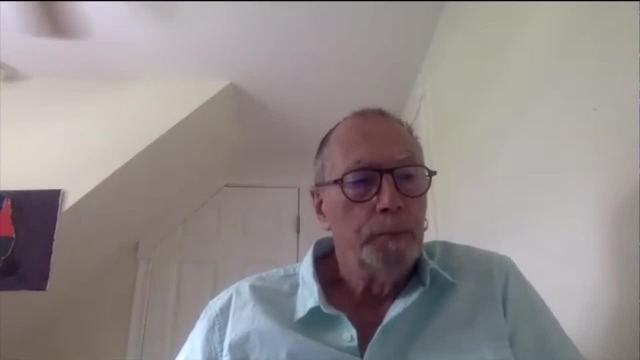 recursive process And recursion theorists call this kind of set recursively enumerable. So if you open a book on recursion theory, if you get a definition of a formal theory, it'll tell you that it's a recursively enumerable set of formulas of some formal language. 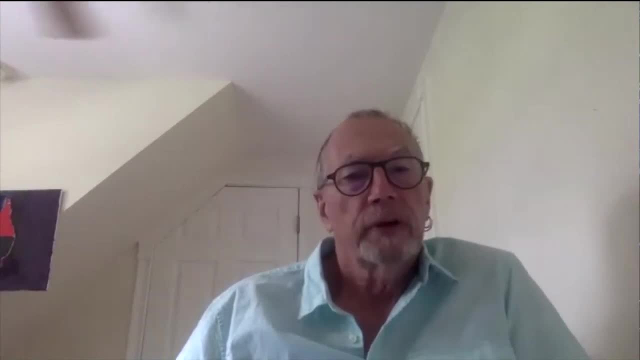 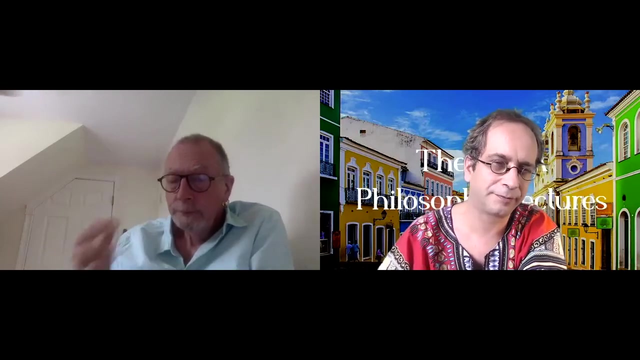 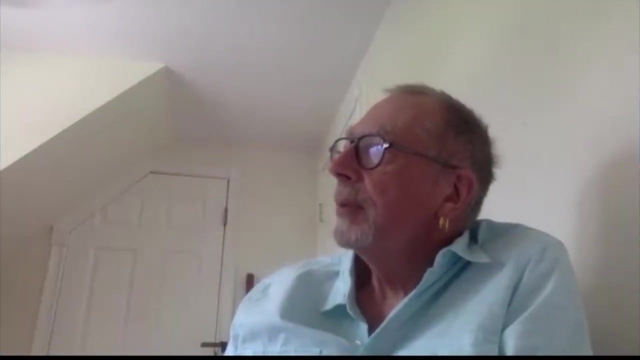 So that's a more abstract setting, And sometimes you will see discussions of Godel's theorem in that setting, that context. Okay, Now to Godel's incompleteness result. What did he show? Well, again, Godel's incompleteness result. 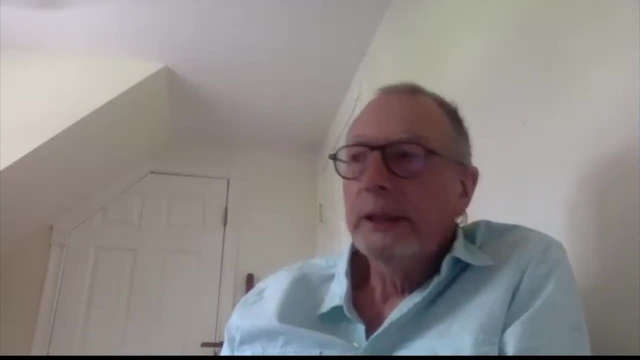 There's standardly two, Okay, And the problem is that each of those can be phrased in different ways as well, So let's take the first one first. What Godel showed was that if you take the standard axiomatization for arithmetic, then 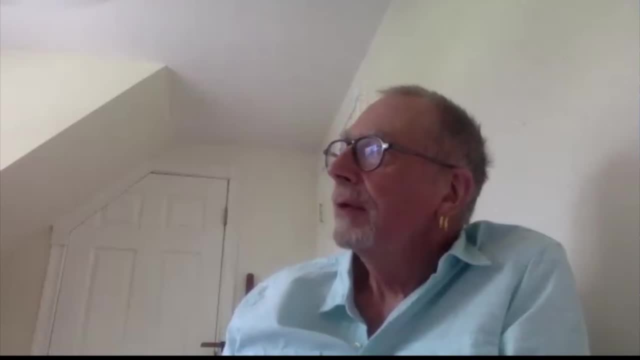 there are things- Okay, Things which are true in the standard model, which are not provable, So it's not complete. If you want to put this in more technical terms, what he showed was that let's come to that in a second. Godel's actual proof used the standard axiomatization for arithmetic. 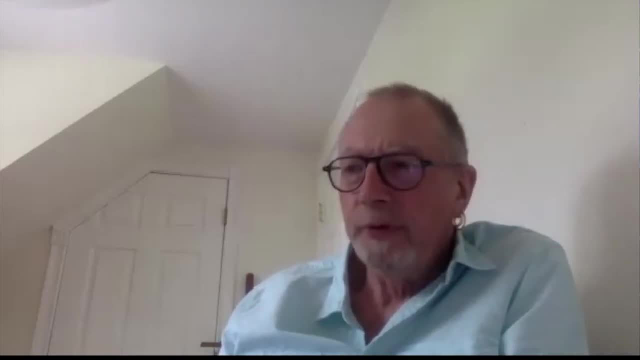 of the day, But it's pretty clear from his proof that it's going to apply to any axiomatization. Okay, So the standard axiomatization was incomplete, but it was clear that you know if you tried to beef it up by adding extra junk, you're going to end up in the same situation. 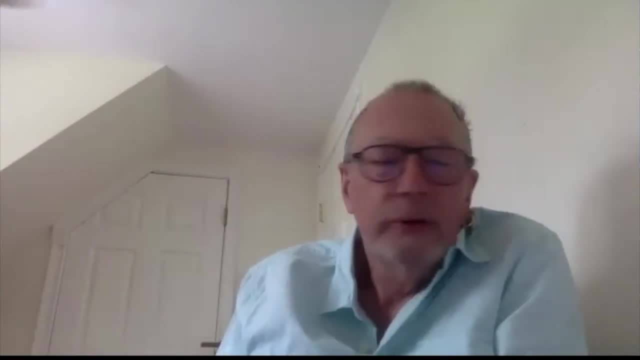 So what he showed was that you just can't axiomatize the set of sentences which are true in the standard model. And, if you want to put that in more abstract terms, what he showed was that the set of truths in the standard model of arithmetic is not recursively enumerable, because to be 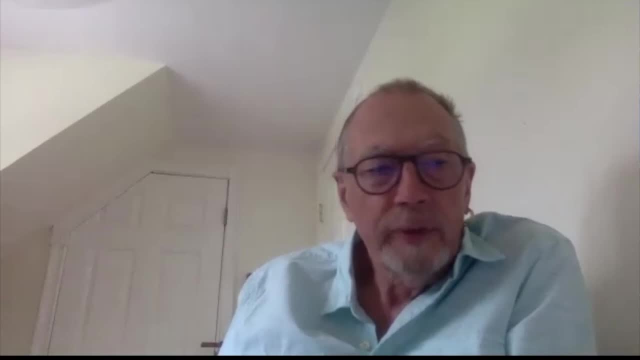 super new. it just has some axiom system or other. So this is the most abstract way of looking at his first incompleteness theorem. You can't axiomatize arithmetic. Now. remember Hilbert's program had two parts. The first was: let's axiomatize mathematics, in particular arithmetic. 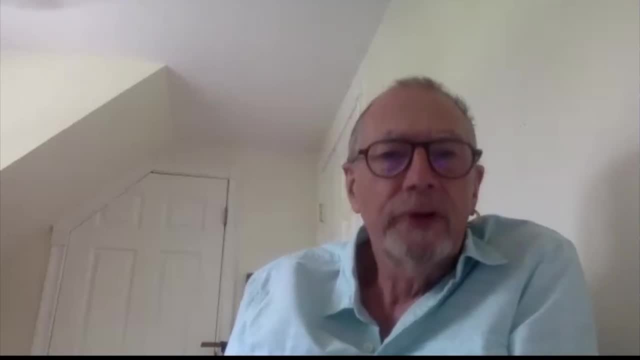 And then, when we've got that, then we'll prove that it's consistent by finite remains. So Gödel's first incompleteness, theorem G1 as logicians sometimes call it- was that you can't axiomatize arithmetic. Okay, 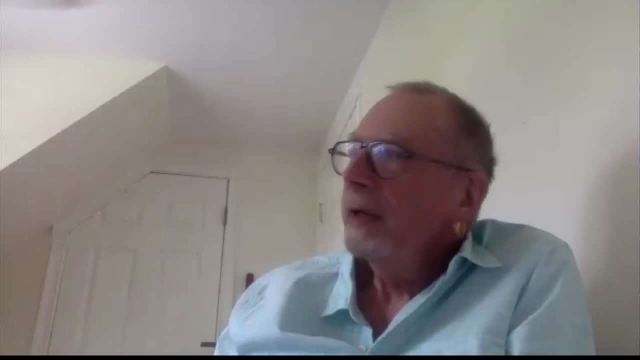 That's one nail in the coffin. but the second incompleteness theorem G2, said that if you take the statement that that theory is consistent, Then it's kind of interesting. but you can actually formulate that as a statement of arithmetic itself. 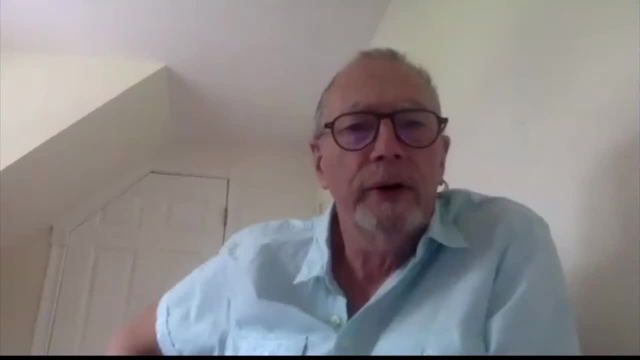 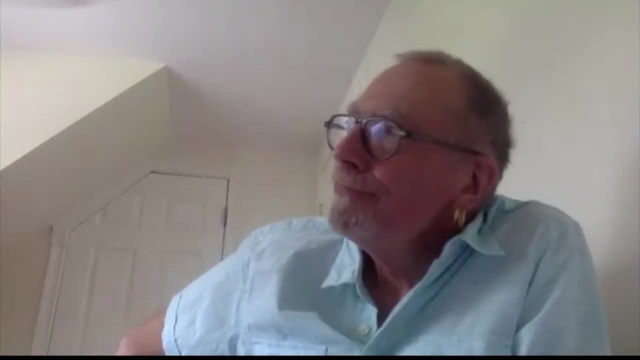 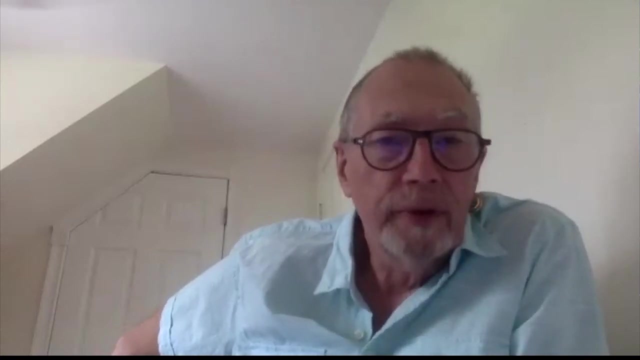 It's not obvious, but one of the cool things that Gödel did was show how you could express statements like that in a certain sense in arithmetic. So proving that your axiomatic arithmetic is consistent is proving a statement of arithmetic. And what G2 shows. 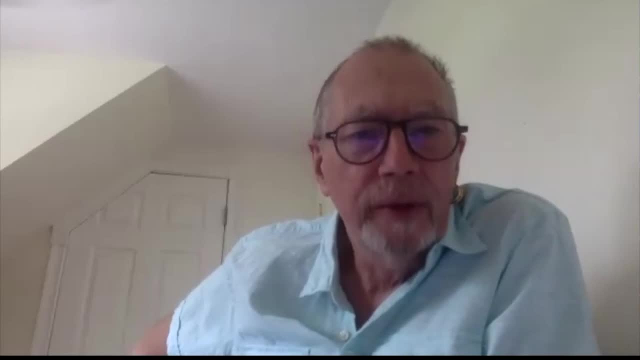 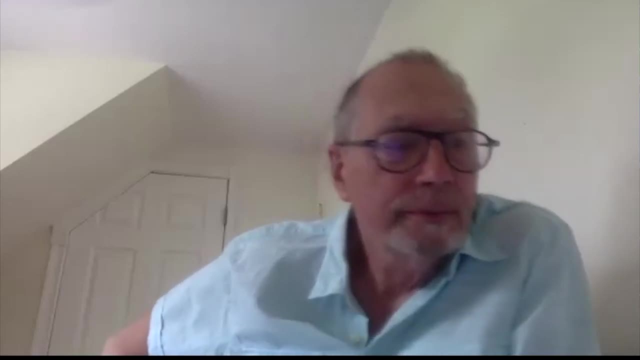 Okay, G2 shows is that you cannot prove this statement. So from the first theorem we knew there were things which are true in the standard model which are not provable. The consistency of the arithmetic is true in the standard model, but it's one of these. 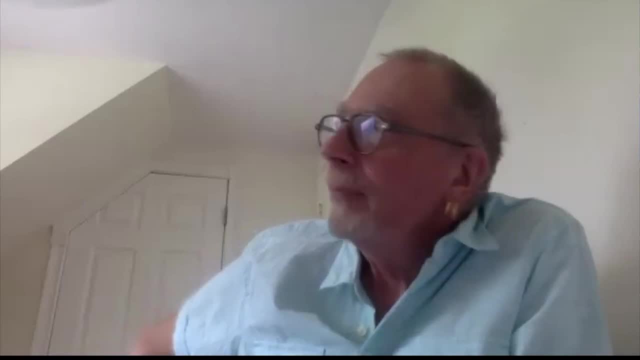 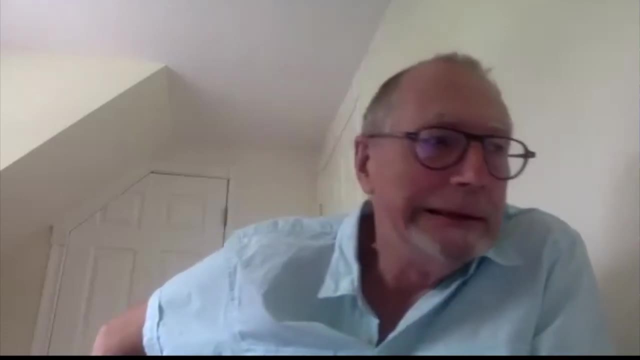 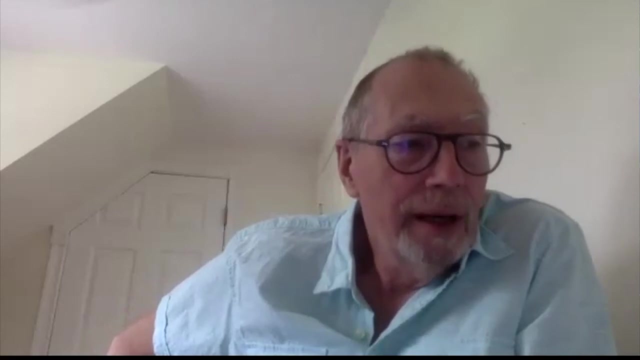 things you can't prove. So if you can't prove it in this arithmetic, you certainly can't prove it in the finitary part of it. So that was the second nail in the coffin: You haven't got the axiomatic, You haven't got the axiom system and you can't prove it consistently in a finitary. 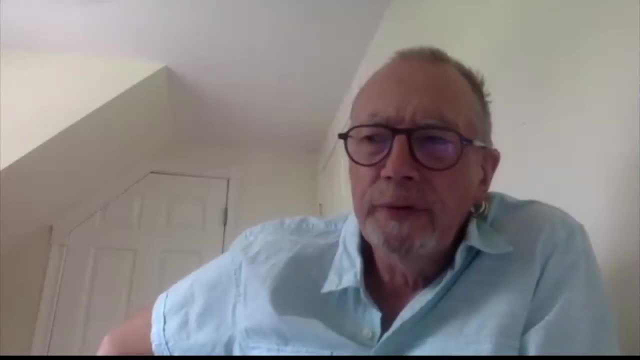 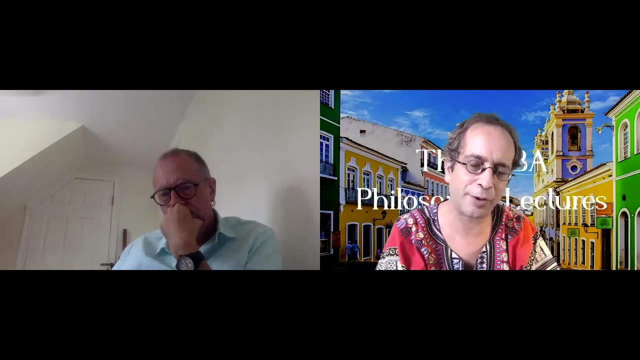 way Okay. So that's the sort of rough and ready discussions of Gödel's two incompleteness theorems. In popular formulations, the incompleteness result is sometimes expressed in by saying that: So you're saying that there are truths in arithmetic that cannot be proved. 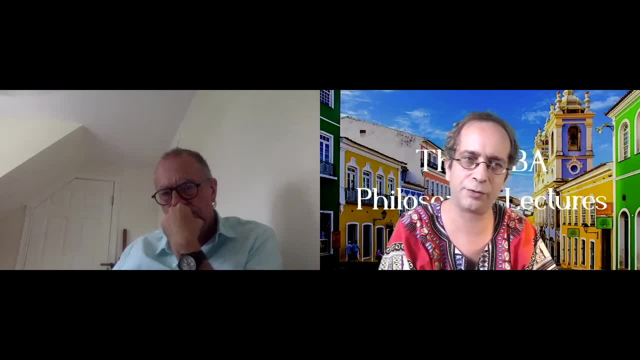 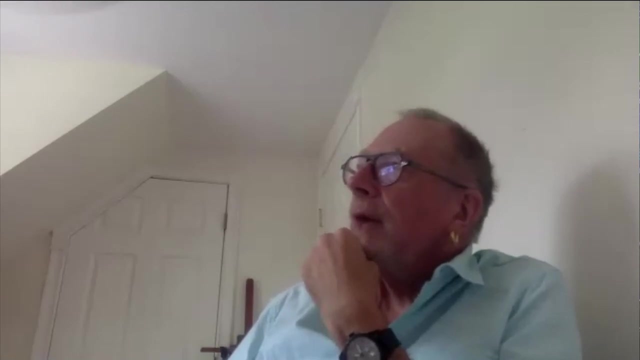 But probably a better way of putting it is that if arithmetic is consistent, there are truths that cannot be proved within that system, Correct. So we haven't talked much about the underlying logic of the theory of arithmetic. I mean, standard assignment is not a theory of arithmetic. 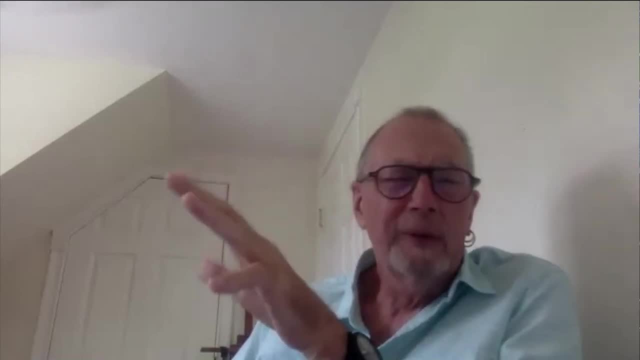